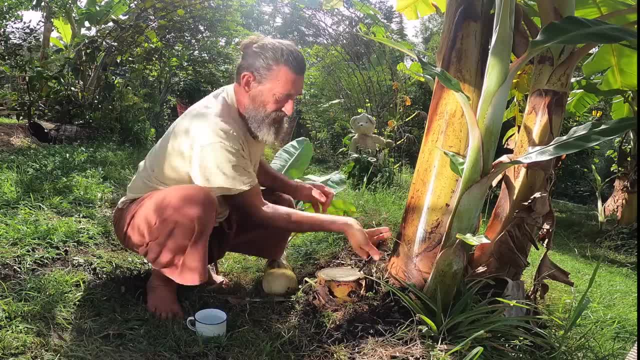 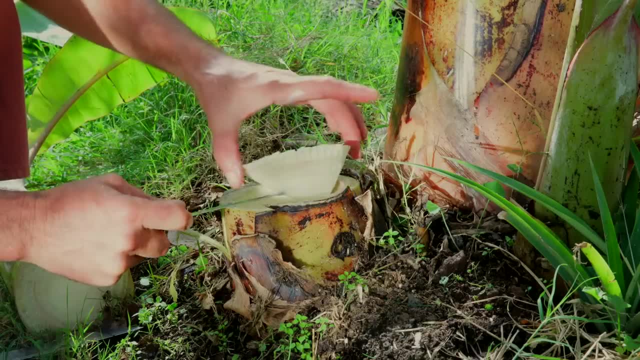 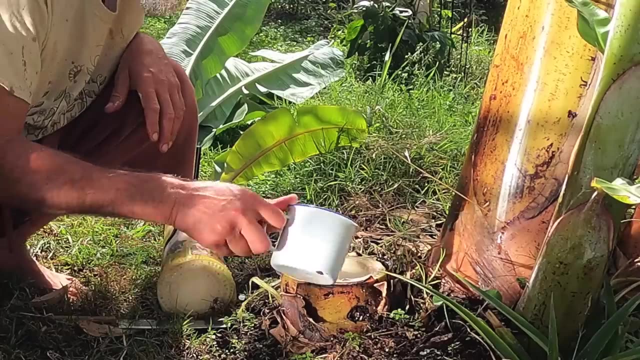 Sort of cut the middle out of it like a bowl. see All the way around, And you should be able to just pop that out. see Just like that. And then all you need to do now is put your water in and it won't come back and that'll rot. 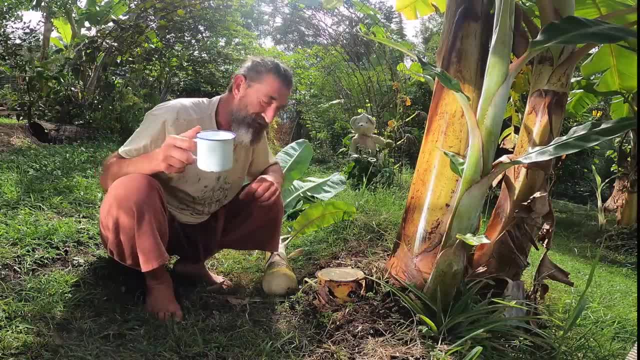 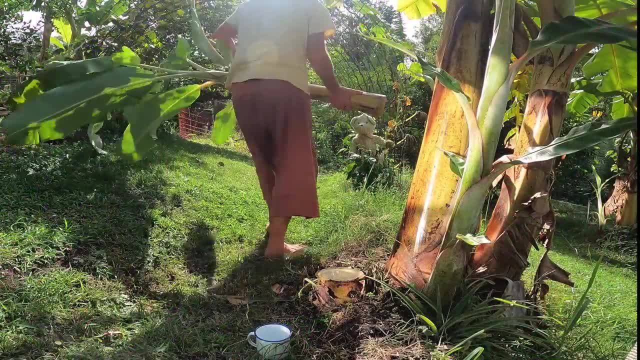 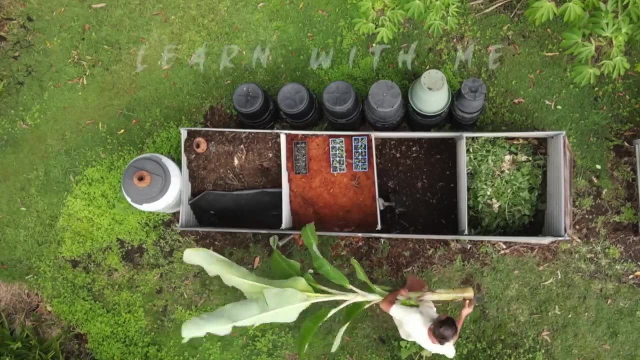 And that's a much cleaner, friendlier way to do it. It doesn't cost anything. Okay, I'm going to put this one in the compost now. There we go. So I want Weedy Garden Channel to be a channel where you can come. 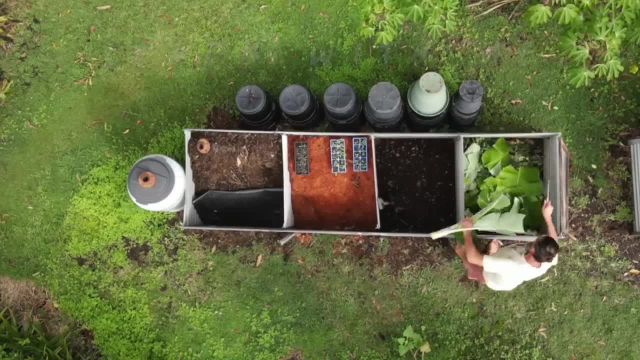 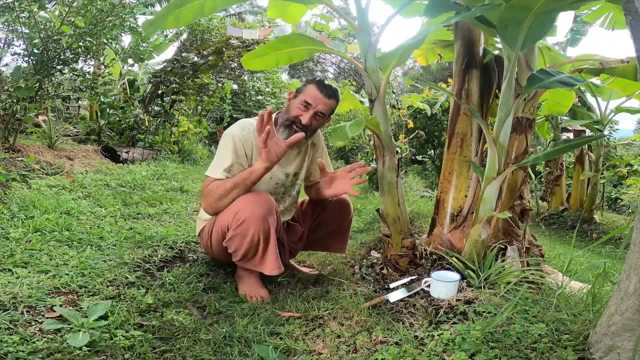 and learn all sorts of stuff about all sorts of things to do with gardening and permaculture and organics, And it's not only what I can share, but it's what you can share as well, And on this video I'm going to share some things that you've shared with me. 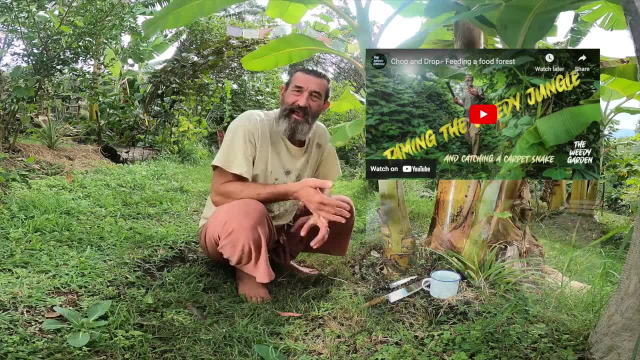 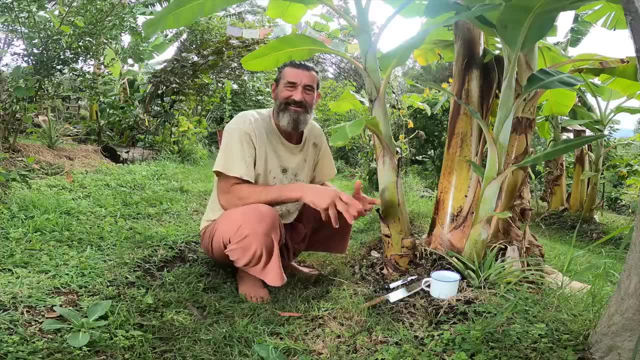 I did a video- this one here- about 12 months ago, And in that video I showed that I was chopping my banana pups out, But I was complaining that they kept growing back. So I kind of asked: does anyone know a good idea? 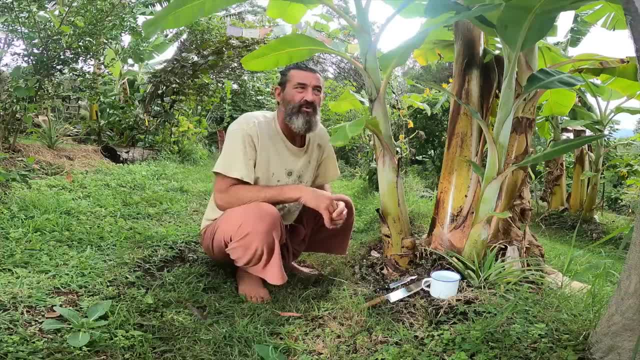 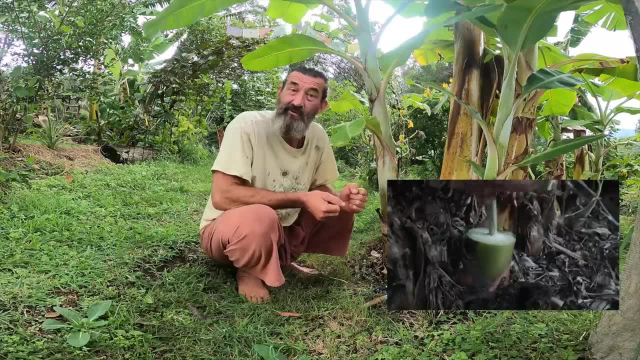 And I got a message from one of my subscribers who I think grew up in a banana plantation. She said that when they chopped them out they stuck a stick in it and put some kerosene in it or diesel, like I explained. 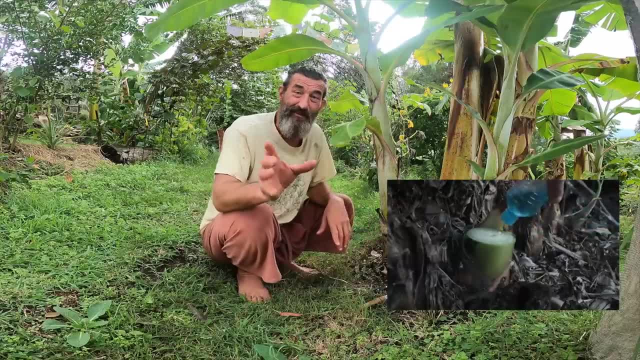 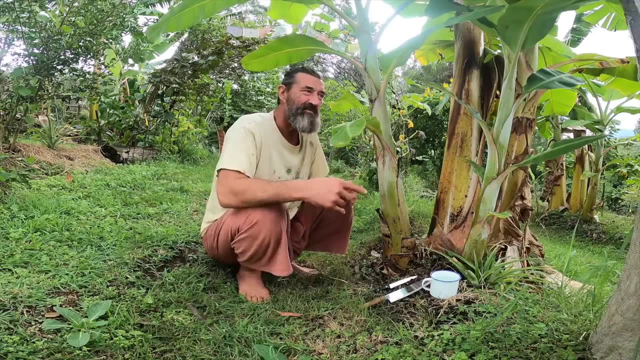 And it kept them from growing up. And, I must admit, my initial reaction was, oh no, I'm not going to do that. But then I thought, okay, well, if they've been doing it and they keep doing it and the bananas keep growing. 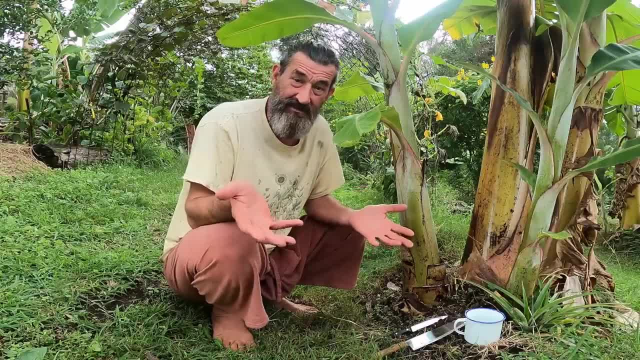 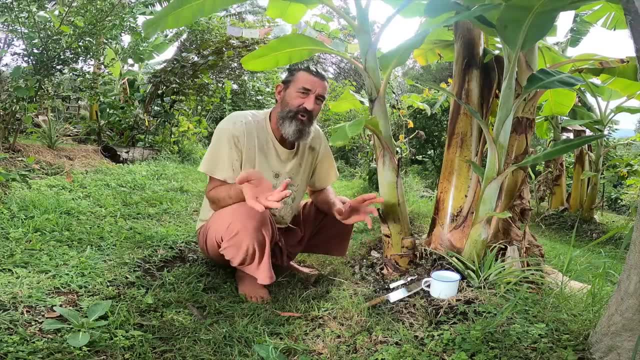 then it's not going to hurt the bananas. I didn't know any other way to stop the banana pups. So I kind of felt like, okay, I'll do that and I'll show that and I'll share that. That was a bit controversial in the organic circles. 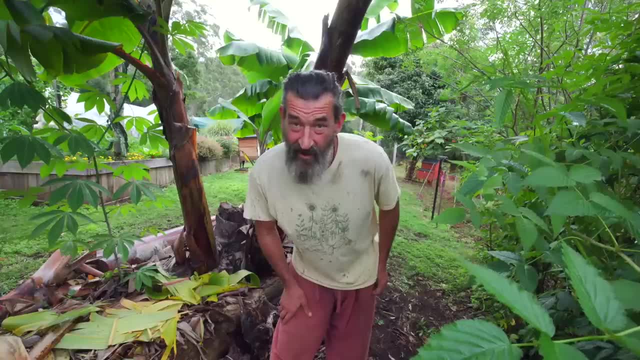 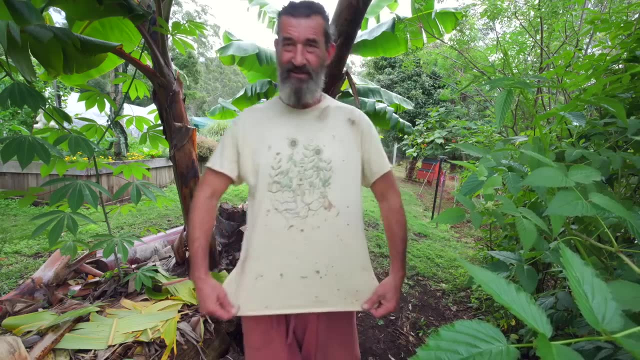 See, okay, let's move on. Okay, another really good thing I learned since I did the last video is that banana juice really stains your clothes. So you can see my Wheatie Garden t-shirt. See all these stains on it. 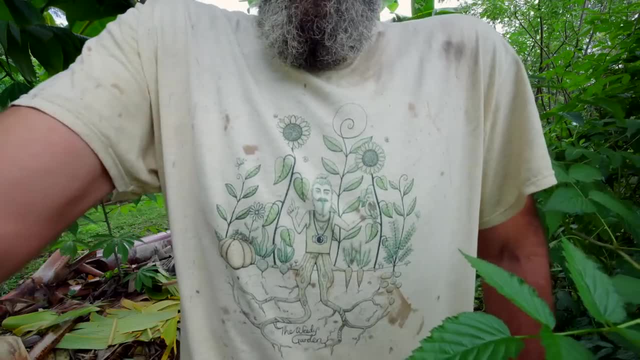 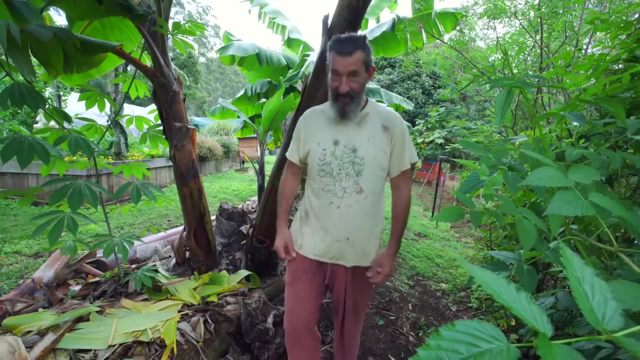 I've already washed it twice. They're all permanent. now I don't know if you can see that, but that's dirt. That's from this morning. But banana juice- you won't get that out again, so use your old rags. 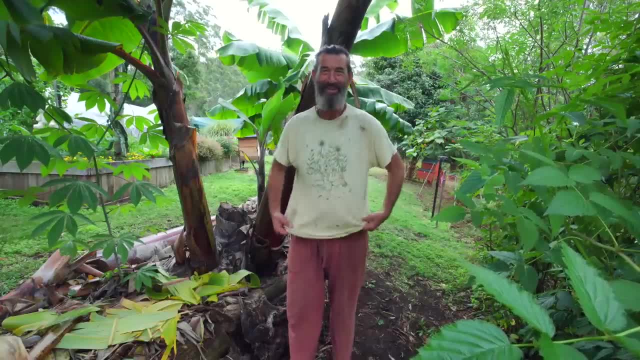 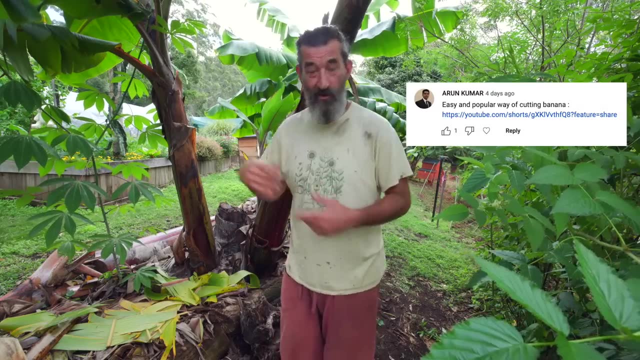 Or just use the Wheatie Garden t-shirt and buy another one. Okay, so one of the earlier comments on my last banana video was someone put a link on that comment. You can see the link in the description of the little short. See that short. 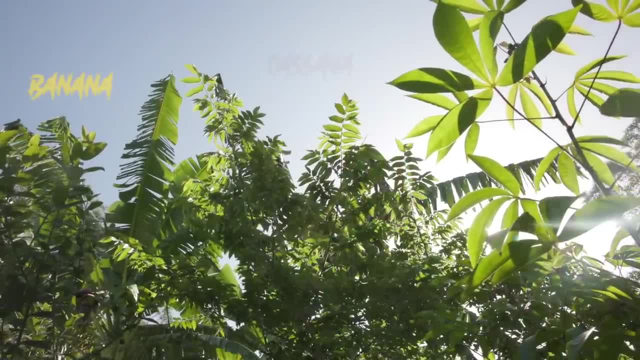 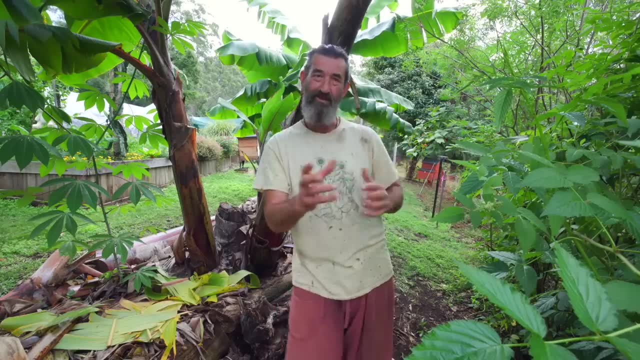 Although it's a good technique if you've got room, I'm a little bit afraid if I do that for some of my banana trees, they're going to crash into some of my other trees that are planted around, because my food forest is kind of pretty compact. 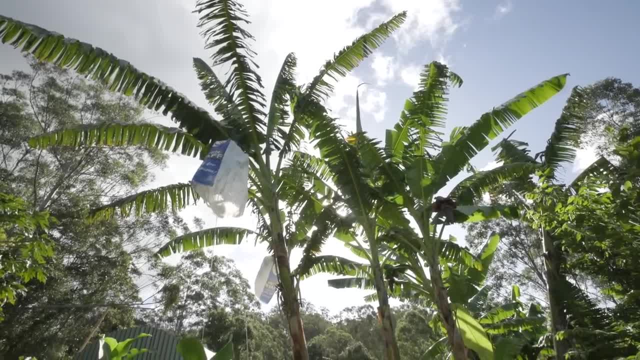 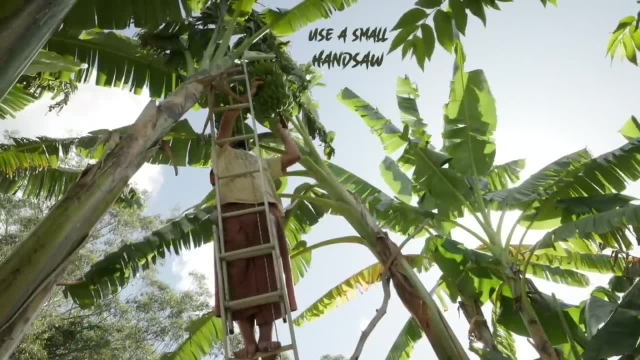 So until I think of another way, I'm going to continue climbing up my ladder Using my long knife. I can trim the leaves down one at a time, and then I can slowly take the tree down. But the thing I like about the Wheatie Garden channel is the stuff I'm learning. 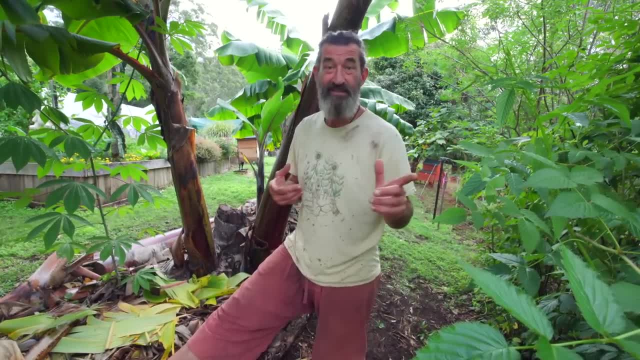 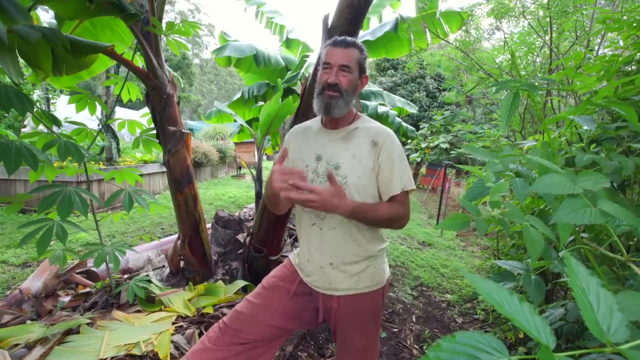 The comments below in all my videos is people come with really good suggestions and that's how I learned that little trick about the water and the banana pup. So if you do have any comments, any good suggestions on any themes that I'm doing in my videos, 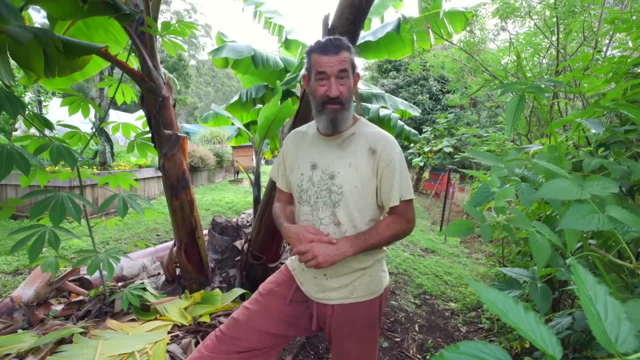 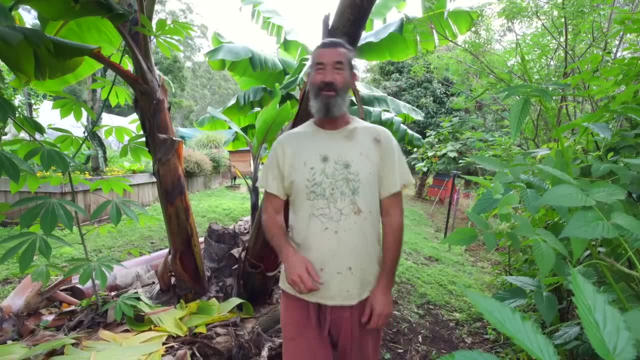 please put them down. Don't feel like Wheatie knows everything, because Wheatie doesn't know very much at all. Wheatie's learning most of this stuff from you guys and your comments. Okay, so be nice and share your love and share your knowledge with everyone else that watches the Wheatie Garden. 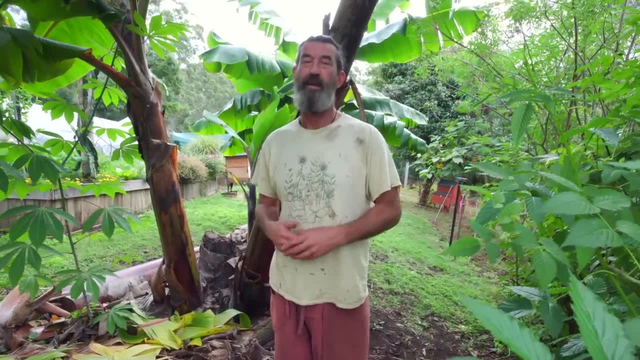 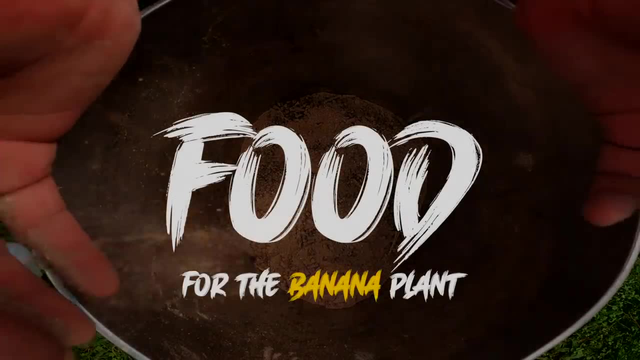 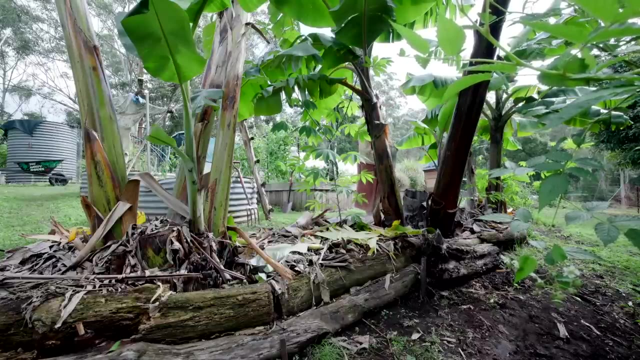 not just me, And some of the good stuff I'll put into videos, like I did today. And so what else have we got going on? I've said banana plants are hungry and they're very hungry, And although I'm feeding them their own great-grandmothers, they still like a lot of extra food. 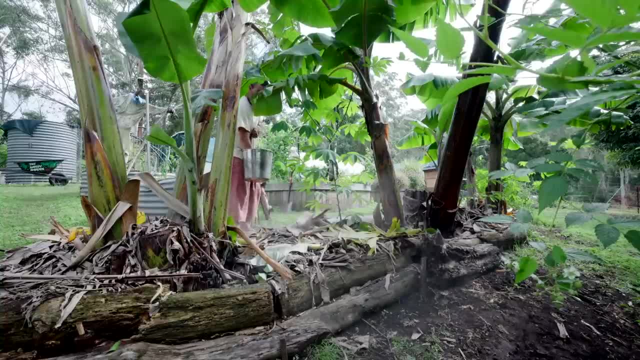 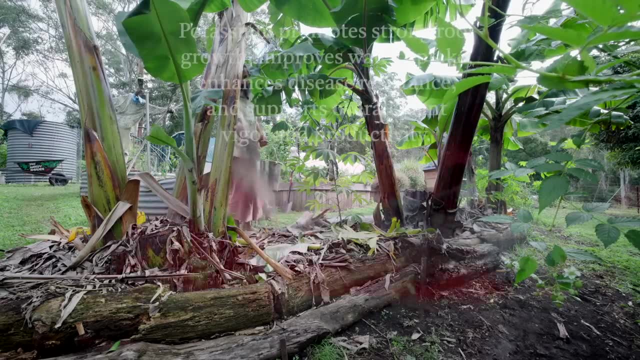 So in this handful here I'm spreading around most of it's ash. We're starting to get a bit cold here in the northern region, So I'm burning my wood fire at night time now, So we've got a fair bit of ash. 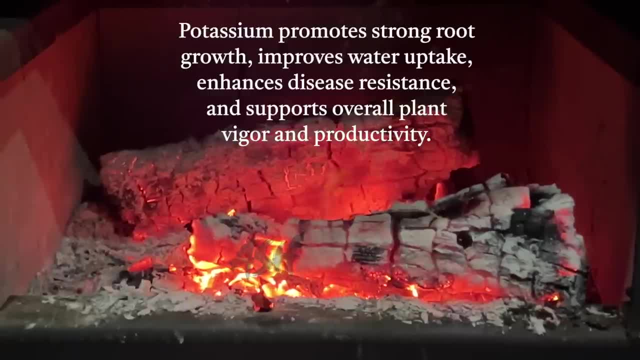 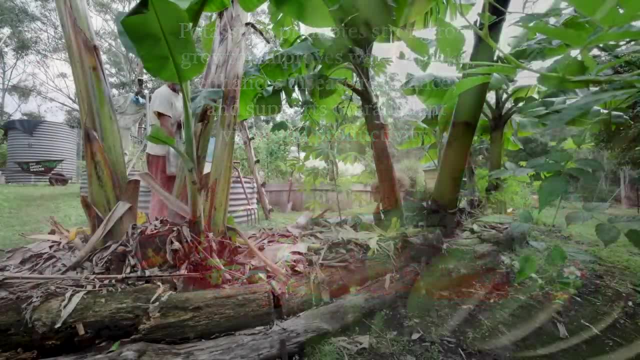 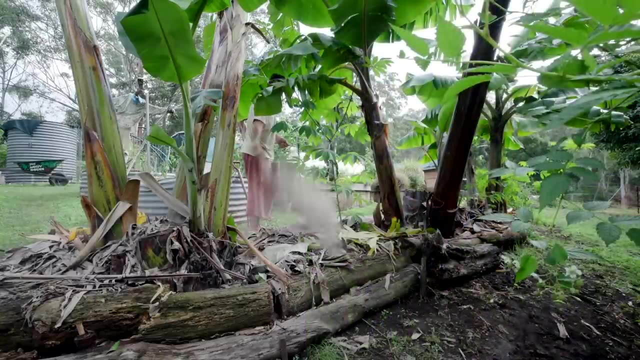 I'll just sprinkle it around the bananas, because there's potassium, as you know. Just Google. why is ash good for the garden? Helps make big bananas Because they're hungry. I've also got a bit of blood and bone in here, because this is not a real jungle.